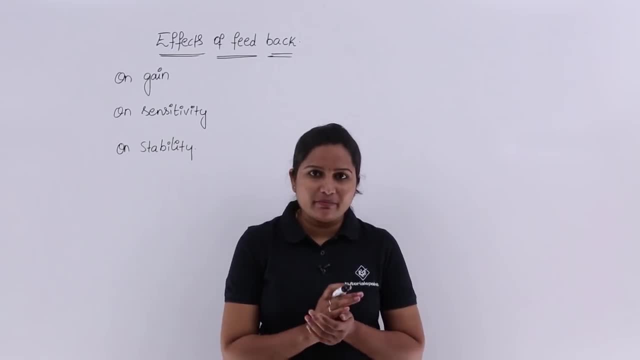 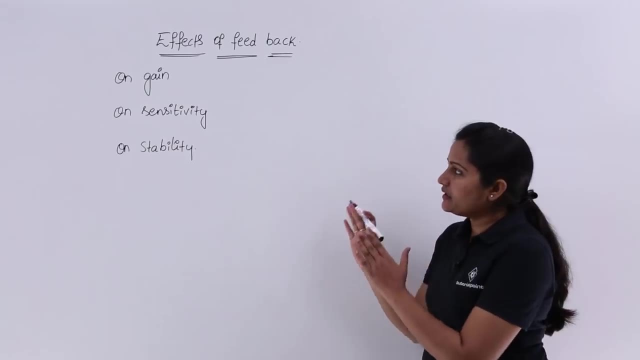 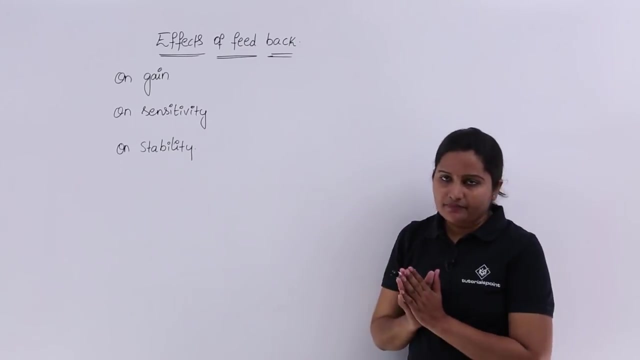 In this video we are going to discuss effect of feedback on control system. So here we are having effect on gain, sensitivity and stability. these are the main effects due to feedback. So on control systems, gain, sensitivity and stability. So here the overall gain of the 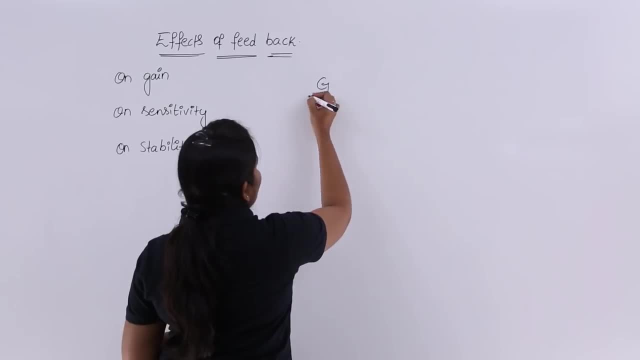 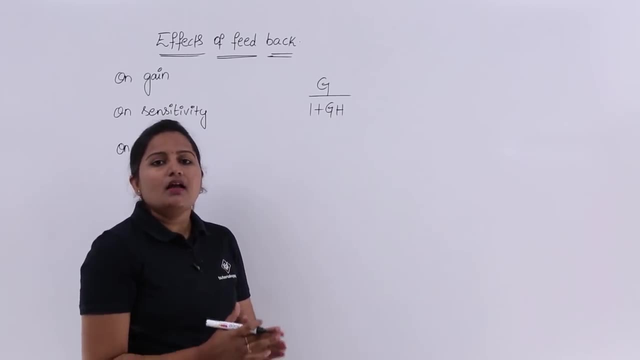 system can be described by the equation transfer function, equation g by 1 plus g h. This is the transfer function or overall gain equation for the negative feedback control system. This is the transfer function equation for negative feedback control system, which shows the overall gain. So if you observe this equation, so this overall gain is controlled. 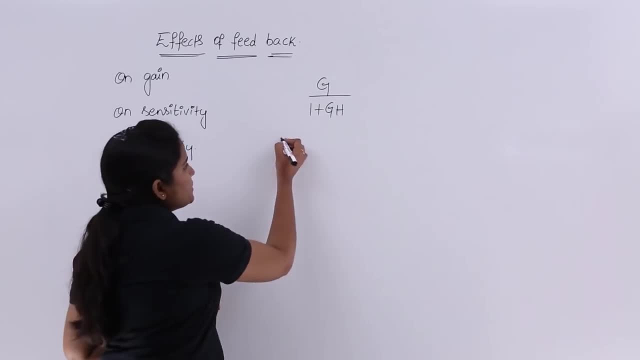 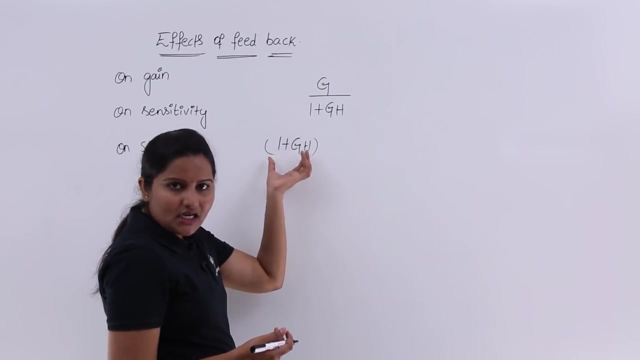 by the factor 1 plus g h here. So 1 plus g h, if increased or if it is greater than 1, than this value is going to reduce if it is increasing. if it is increasing means gh is greater than 1 or gh is positive. if gh is positive, this total value is keep on increasing. if this 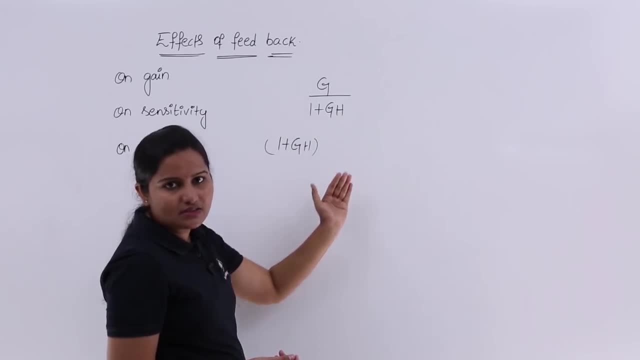 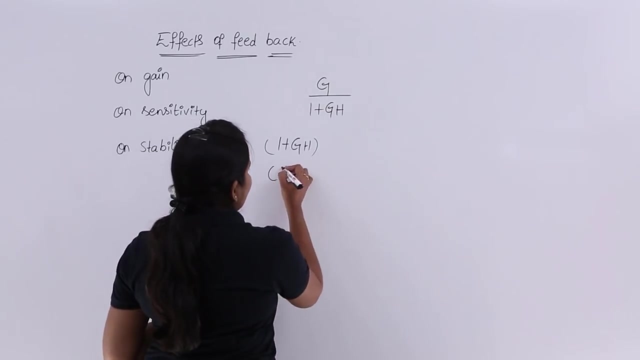 is increasing, the total gain of the system is going to decrease. that means, if you give an positive feedback, if your gh value is negative, then this value will increase. if this value increase means so you are going to decrease your overall gain, so similarly, if you are, if you are increasing this value, overall gain will be decreased. this 1 plus. 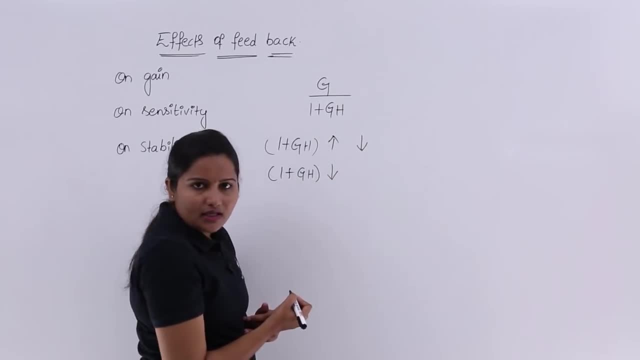 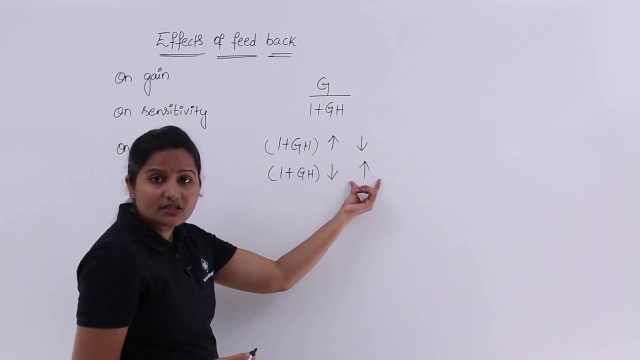 gh value. if you are decreasing, then the overall gain of the system is going to decrease, so the overall gain of the system will increase. the overall gain of the system is going to increase when we will decrease this 1 plus gh value. that means when gh, when gh is a negative. 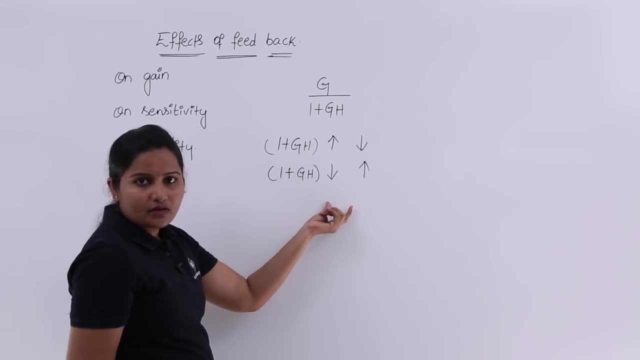 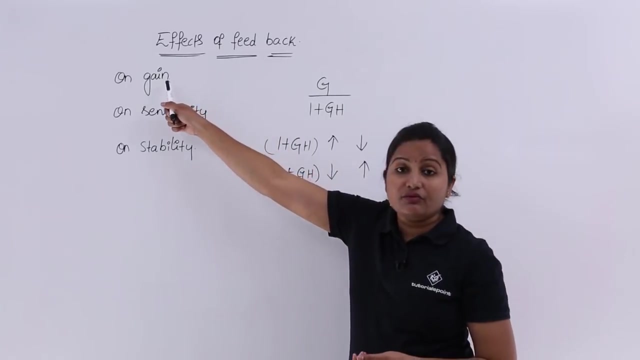 value, then you are going to decrease the value. when gh is a positive value, then we are going to increase the total value. so like this, we are going to affect the gain of this system. like this, the feedback is going to affect the overall gain of the system. if the feedback 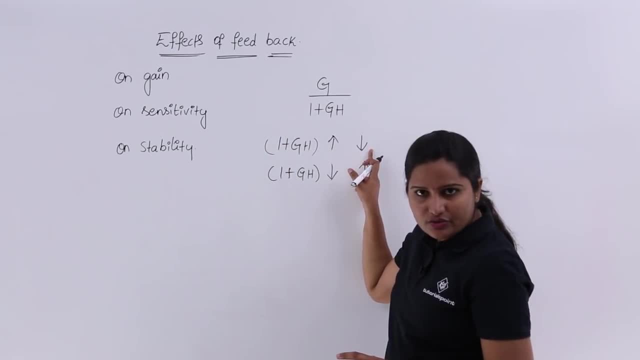 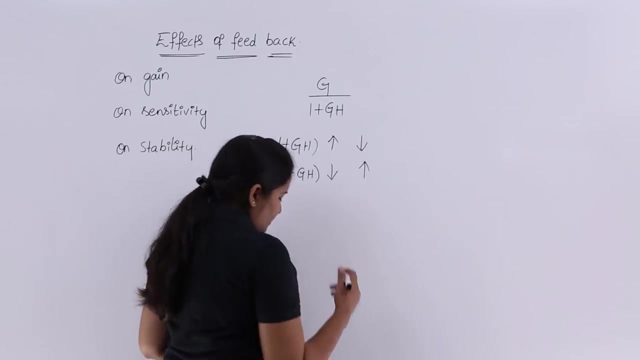 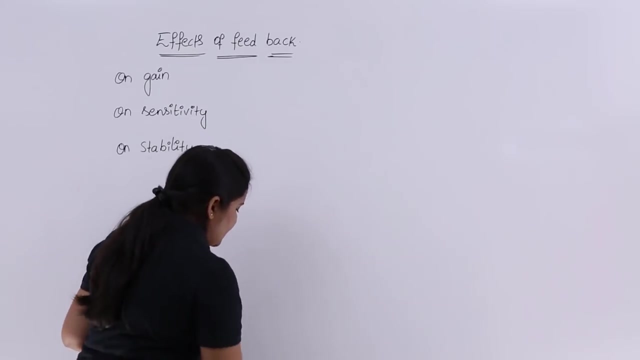 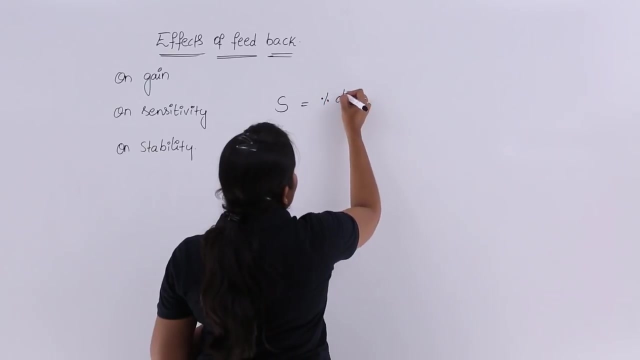 path gain is increased, then total gain of the system is going to decrease. if the feedback gain is decreased, then your overall gain is going to be increased. coming to sensitivity, sensitivity is a factor. it is a very important factor. so here i am going to consider sensitivity as s. this s is equivalent to percentage change in transfer function divided by percentage. 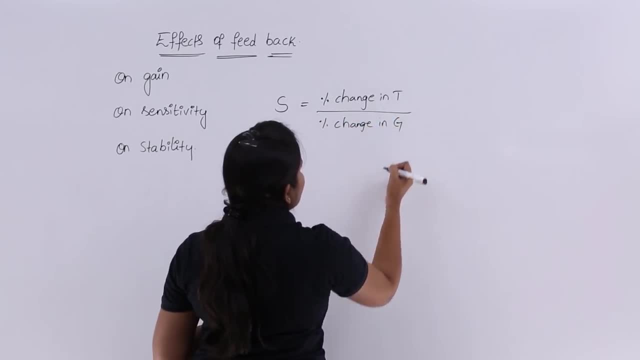 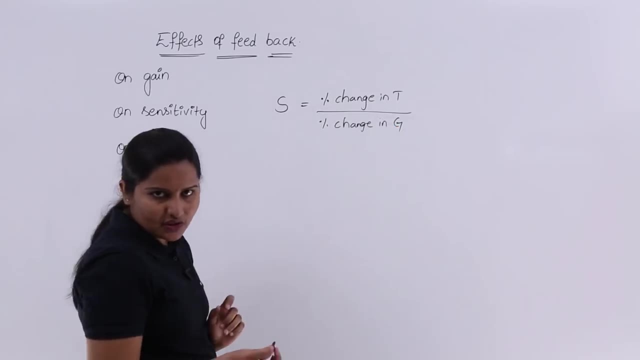 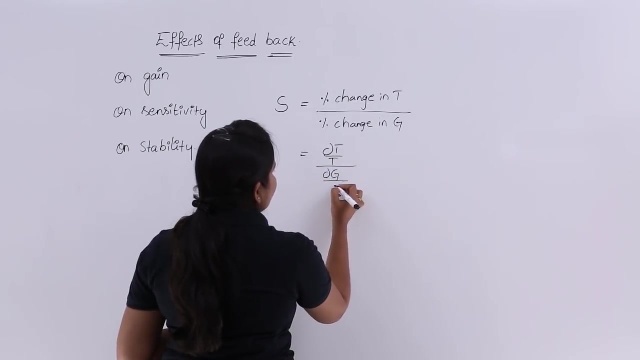 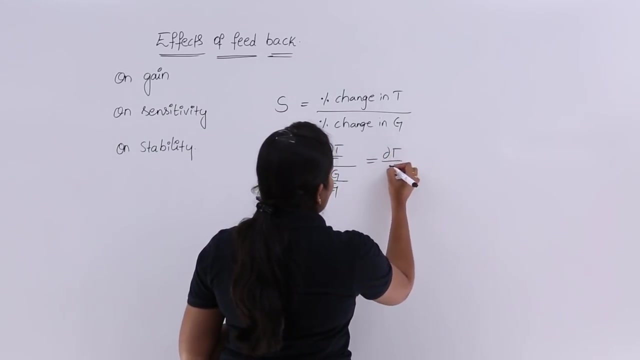 change in gain. we can write our sensitivity in terms of transfer function and gain as percentage change in t divided by percentage change in g. so that means dou t by t divided by dou g by g. so like this we can write so same. I am writing like this: dou t by dou g. 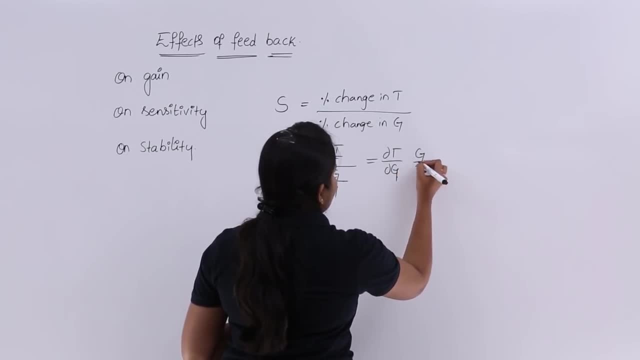 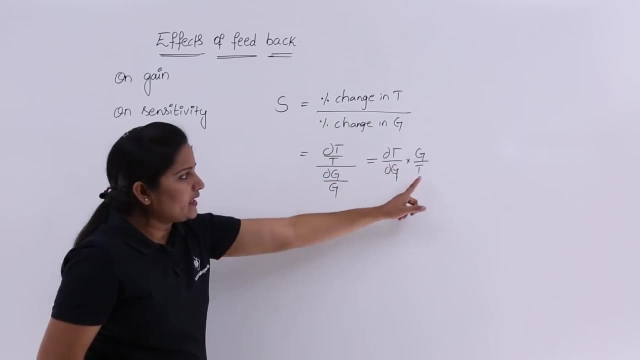 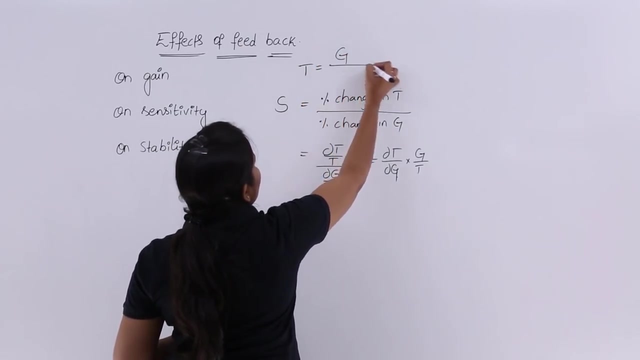 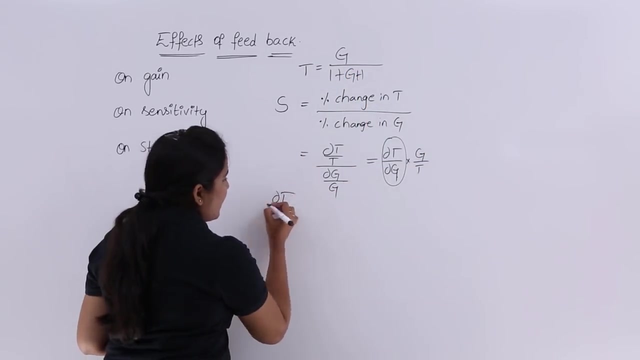 into g by t, you can see. so dou t by dou g into g by t- same thing. I am writing like this: now we know that the transfer function of negative feedback system is equivalent to g by 1 plus g by 2.. okay, I am considering up to here. So dou T by dou G is equal into dou by dou G of. I am substituting: 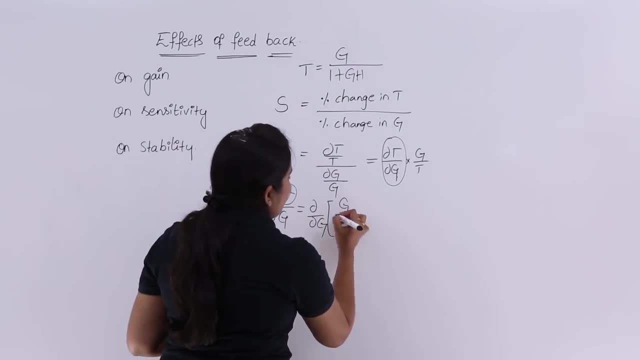 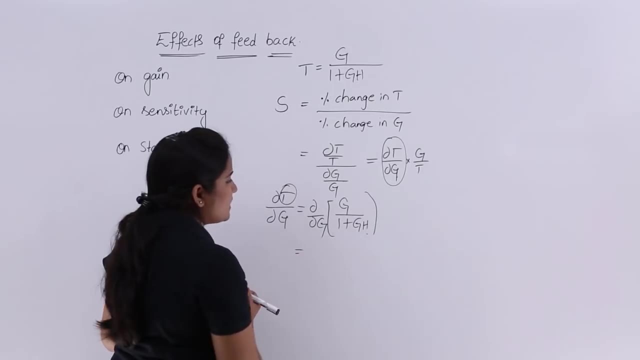 this T value, So now G by 1 plus GH. So how we will do differentiation. So here this is equivalent to V into dU by dV, V into dU minus U into dV divided by V, whole square. 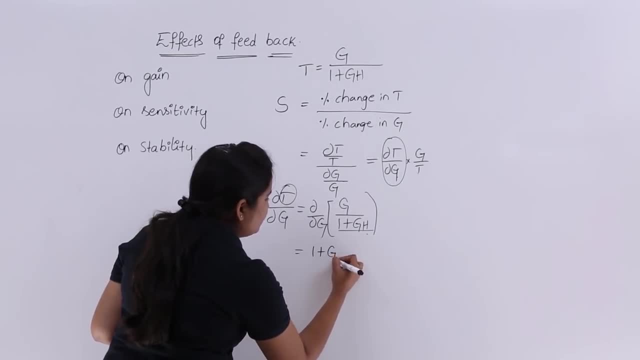 V square, So like that I am doing V into dU. dU means d by dou, by dou G of G, that is equivalent to 1 minus G, into dou V. V is this is in U by V form, So dou V is equal to dou. 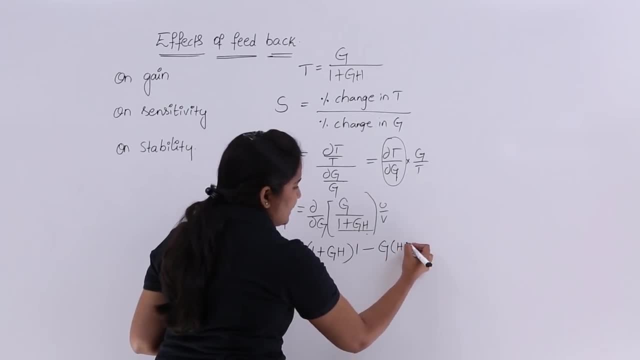 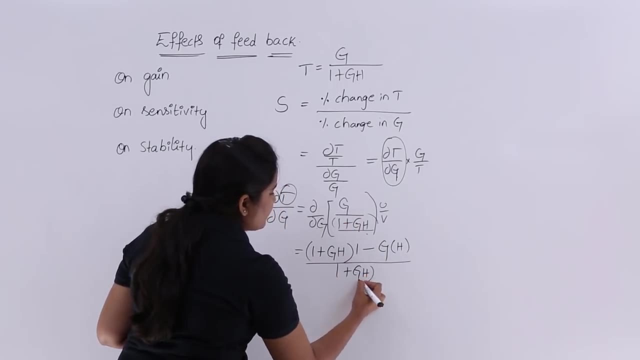 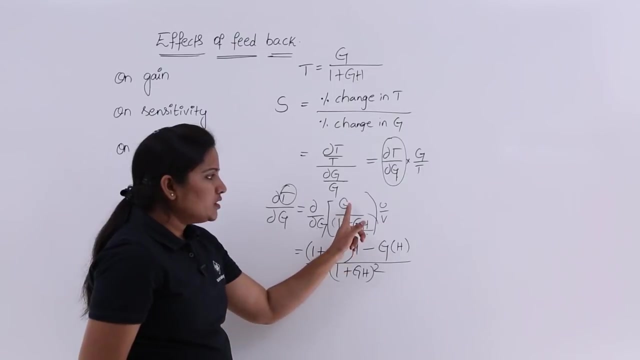 V is nothing but with respect to G means you are going to get H here, and divided by V square means So 1 plus GH whole square. I am treating this as in U by V form. U V into dU. minus dU means with respect to G. if you are doing differentiation, you are going to 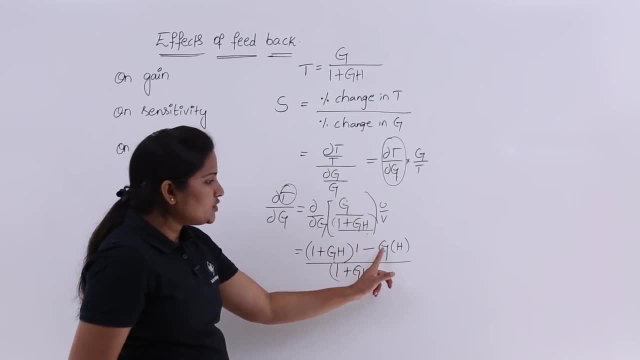 get 1 for G minus U into dV. This is V. 1 plus GH is denominator, So you need to do differentiation for the denominator. then you are going to get H divided by V square. that means denominator square, So this: 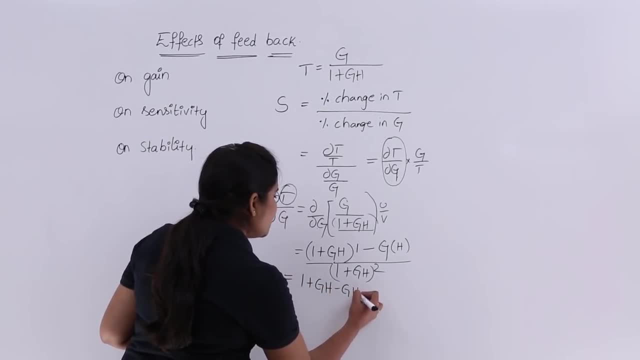 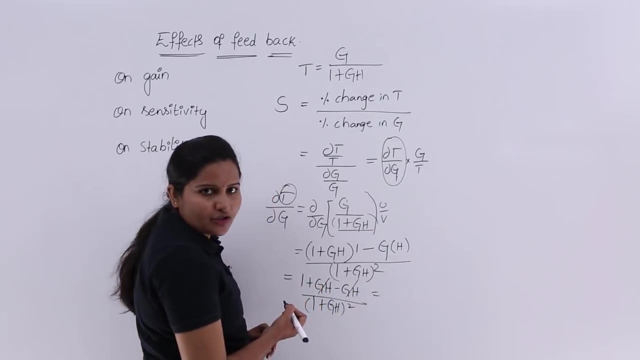 is equivalent to 1 plus GH, minus GH, divided by 1 plus GH whole square. So this is equivalent to GH. GH is going to cancel And we are going to get 1 by 1 plus GH is instead of 1, which. 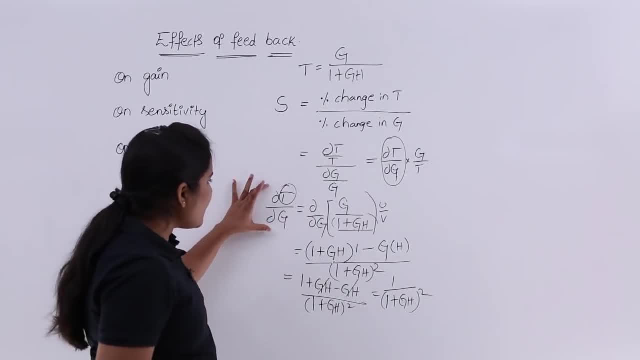 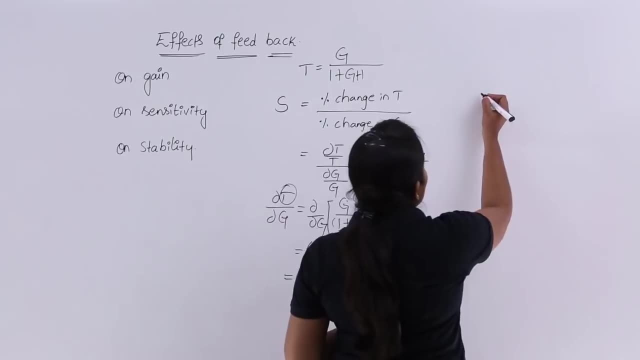 h whole square. So this is the value of dou t by dou g. Now I am going to get g by t value. So what is the g by t value By this? only, I am going to write g by t value as so. 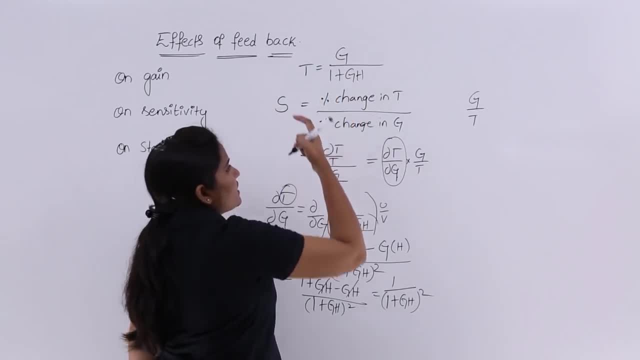 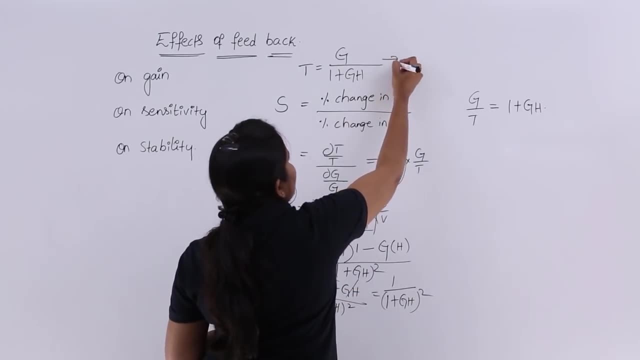 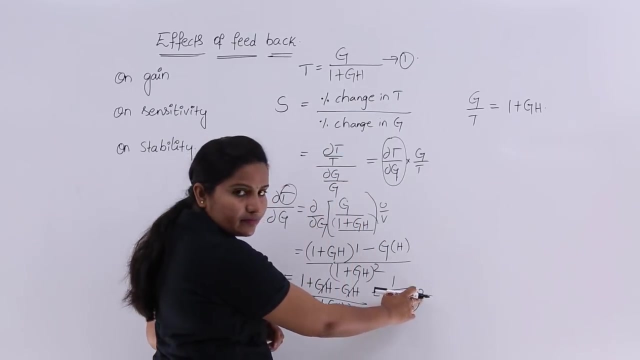 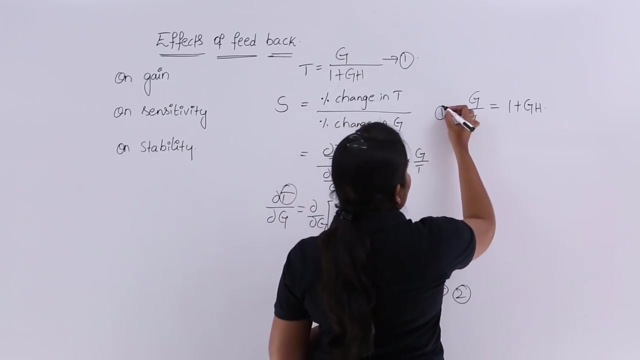 if you send this t to this side, you are going to get g by t value as 1 plus g h. You just consider this equation as equation number 1.. So from equation number 1 only you got this. This you can treat as equation number 2, and here from equation number 1 only you. 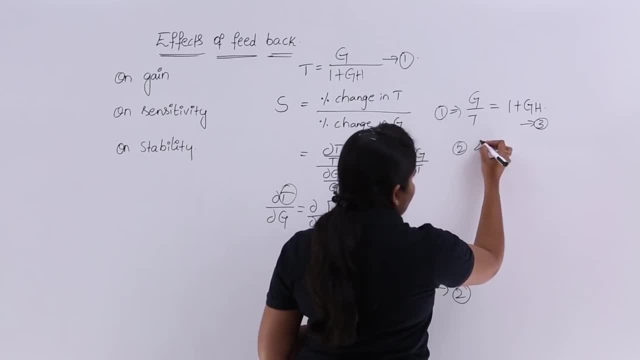 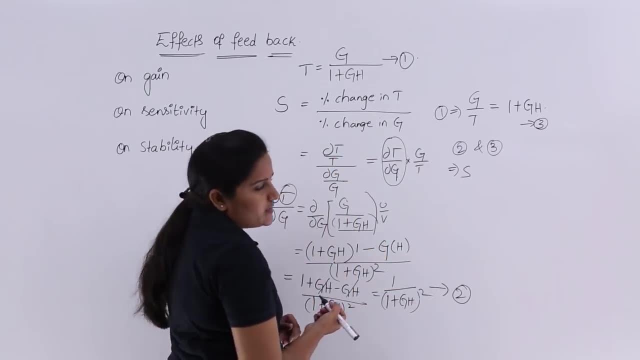 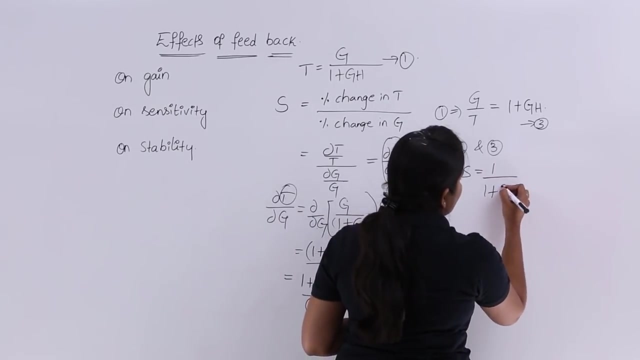 got this equation, number 3.. 2 and 3. you just substitute in S From 2 and 3. your sensitivity value is equivalent to dou t by dou g value. you got 1 by 1 plus g, h whole square. 1 plus g, h whole square into. So here you are having g by 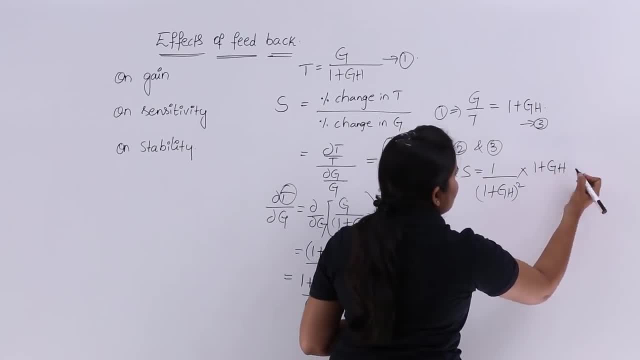 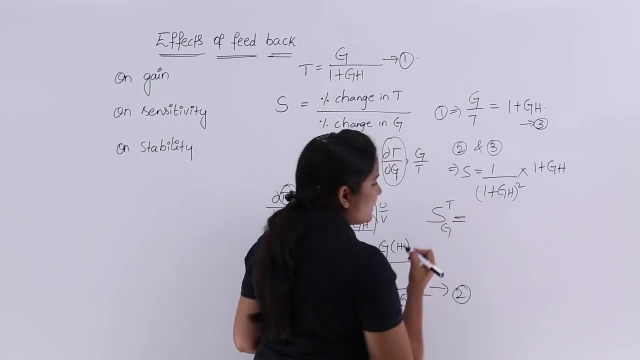 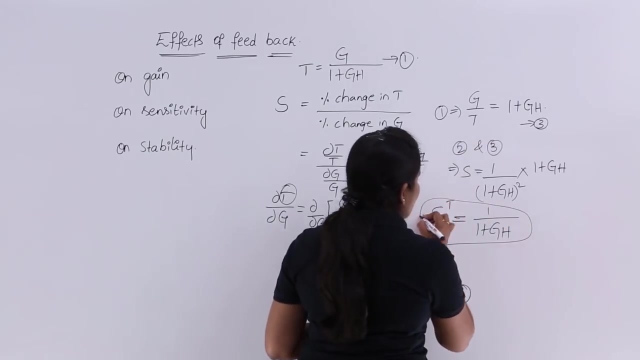 t, g by t is nothing but 1 plus g h. So finally S sensitivity. So sensitivity- sometimes they will represent like this sensitivity- is equivalent to 1 by 1 plus g h. So here sensitivity is also dependent upon 1 plus g h factor. 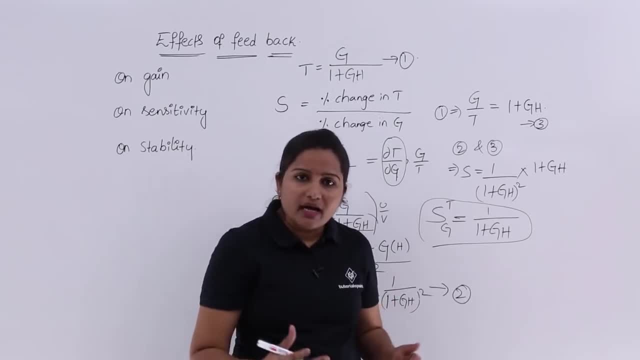 If you are increasing your feedback path value, then sensitivity is going to reduce. If you are decreasing this value. if you are decreasing this value means g h. if g h is negative, then if g h is negative, then your value is going to decrease, Then your sensitivity is going. 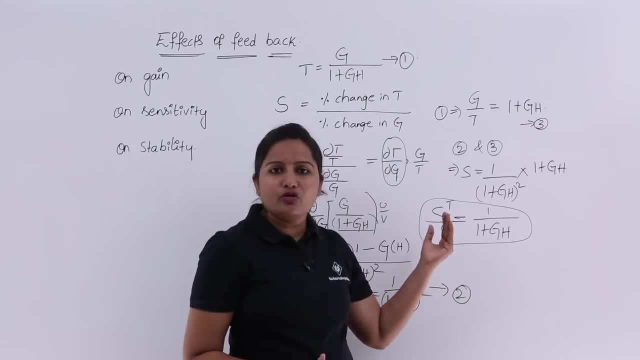 to increase. If you are having more positive value, this denominator is going to increase. total value sensitivity is going to decrease. So here here, the sensitivity is also based on 1 plus g h value. If 1 plus g h is high, sensitivity is going to decrease. If 1 plus 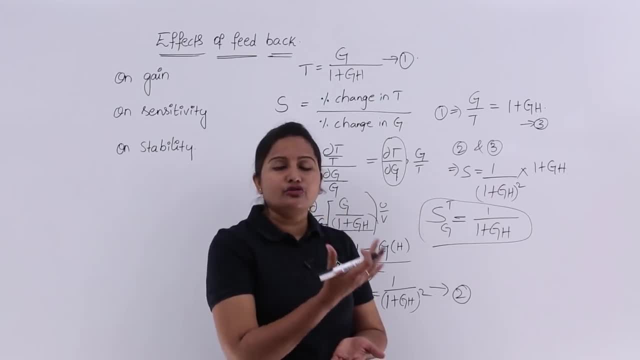 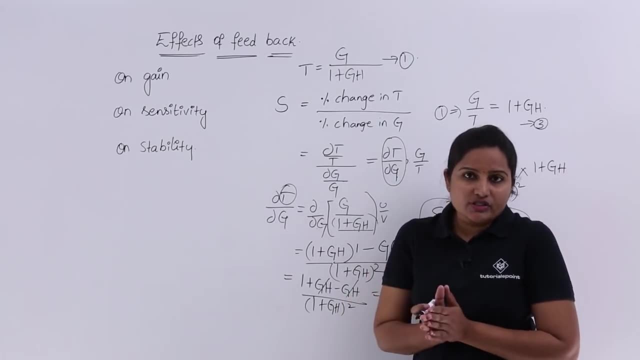 g, h value is low, your sensitivity is going to increase. So, coming to stability, Stability. So whenever your output is stable, then when we can say this system is more stable, whenever output is more controllable, whenever our output is in our control, then we can say that system. 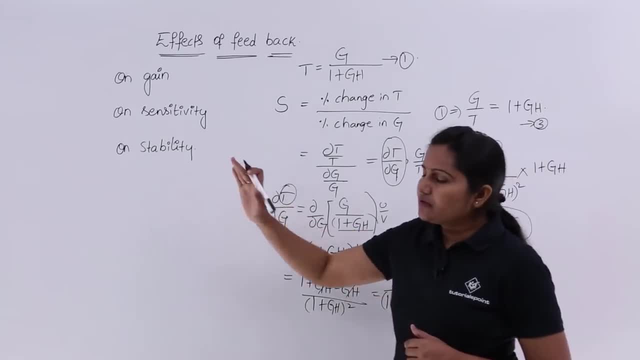 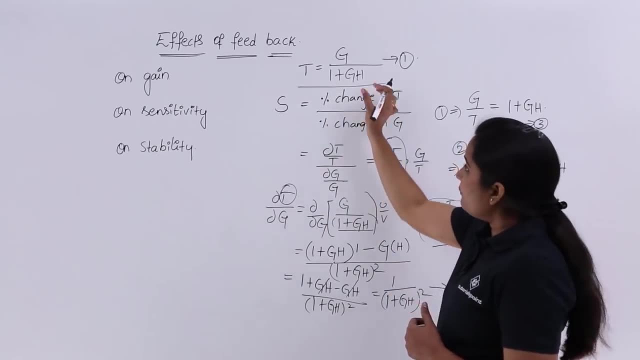 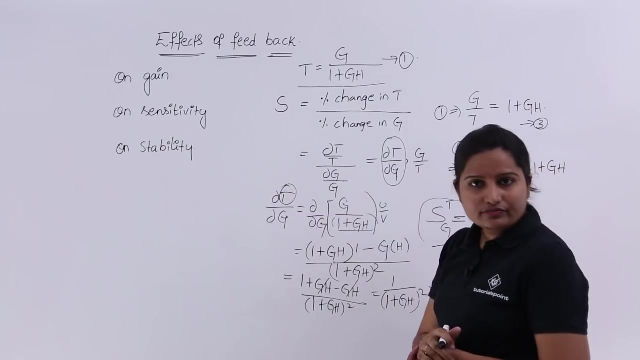 is a stable system. So here, for example, if you are having control system transfer function like this: If your g h value is equivalent to minus 1, what will happens? You are going going to get g by 0, g by 0 is equivalent to infinity. So your overall gain or your 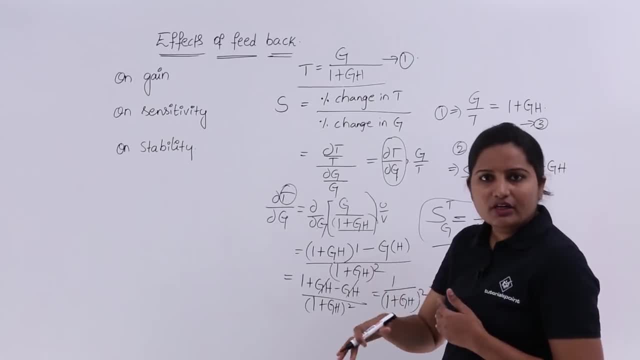 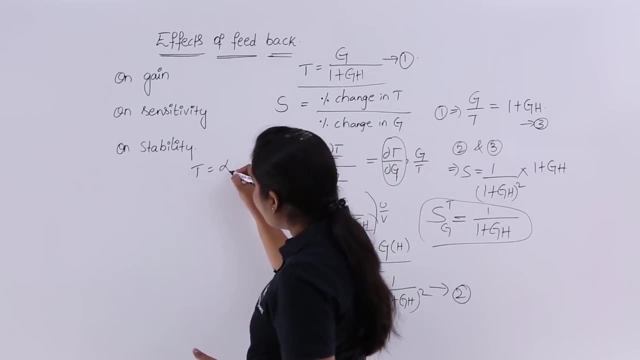 output or anything is not going to be in your control. You are going to get infinity value in your transfer function. If your transfer function is equivalent to infinity, if your c of s by r of s value is equivalent to infinity, transfer function is nothing but c of s by. 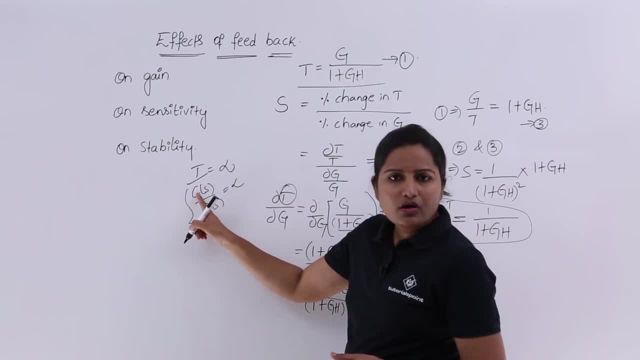 r of s. c of s is equivalent to output transform. r of s is equivalent to input transform. If transfer function is equivalent to infinity, c of s by r of s is nothing but infinity. So that implies your output is equivalent to infinity When you are not having control.